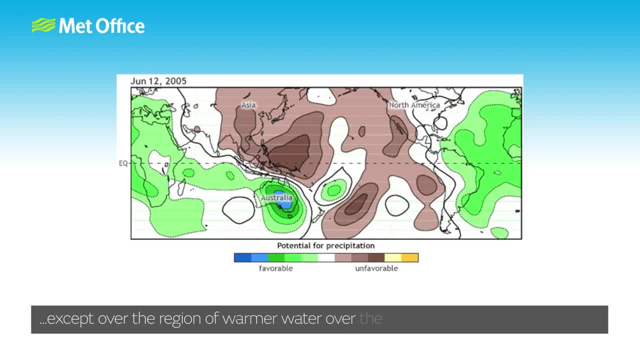 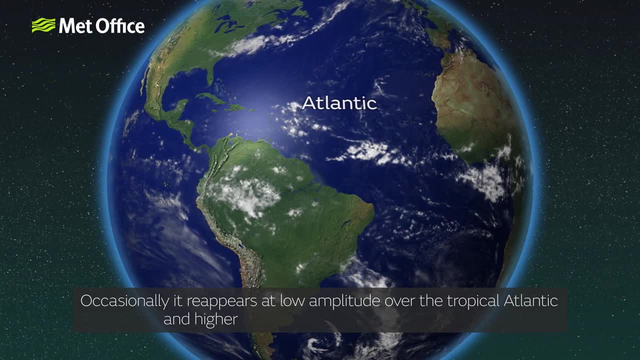 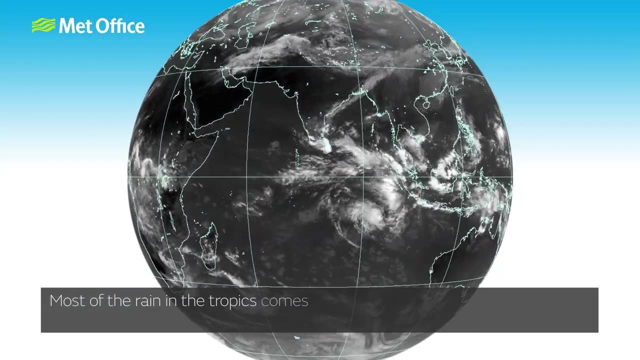 The cooler ocean waters of the eastern Pacific, except over the region of warmer water over the west coast of Central America. Occasionally it reappears at low amplitude over the tropical Atlantic and higher amplitude over the Indian Ocean. Most of the rain in the tropics comes 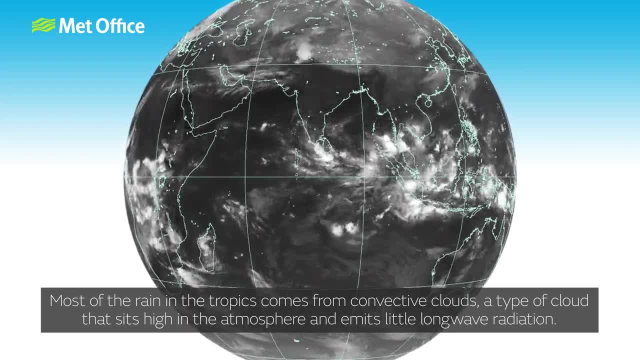 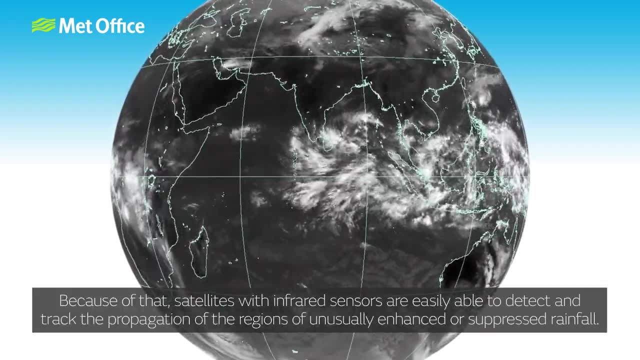 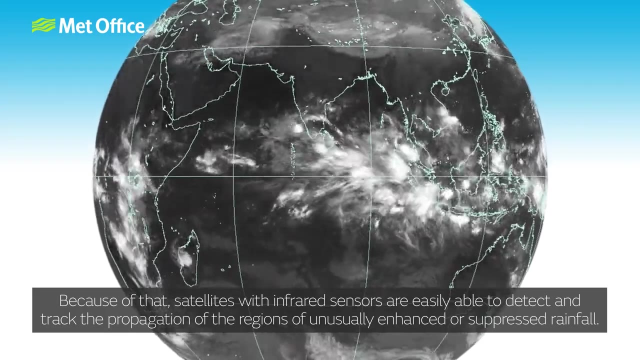 from convective clouds, a type of cloud that sits high in the atmosphere and emits little long-wave radiation. Because of that, satellites with infrared sensors are easily able to detect and track the propagation of the regions of unusually enhanced or suppressed rainfall. The breakdown of the phases is as follows. 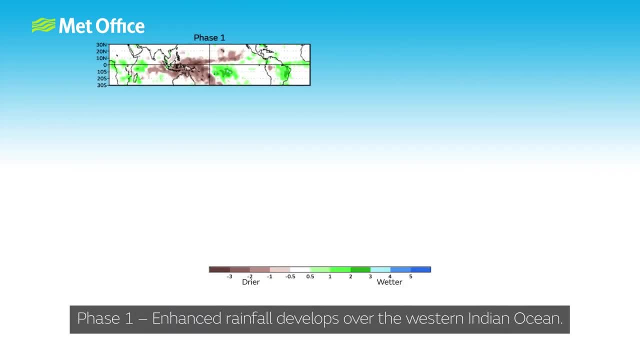 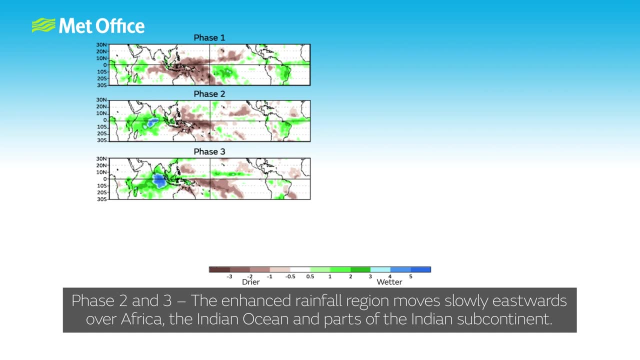 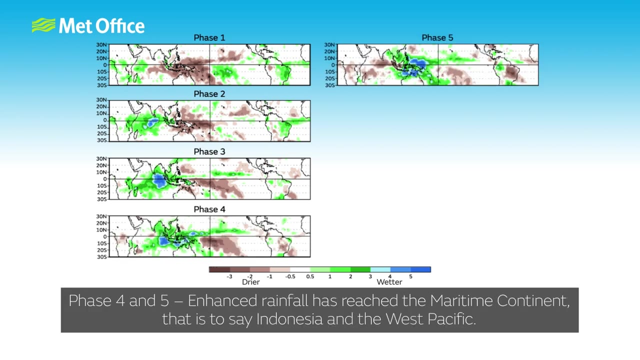 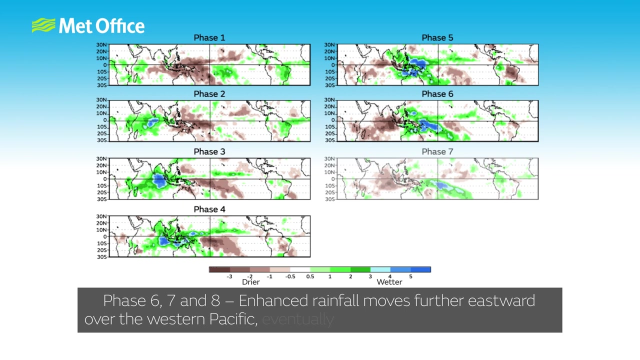 Phase 1: raj dieb. Phase 2: raj dieb, Mopra. Indian subcontinent. Phase 4 and 5 – Enhanced rainfall has reached the maritime continent, that is to say Indonesia and the West Pacific. Phase 6,, 7 and 8 – Enhanced rainfall moves further eastward over the Western Pacific. 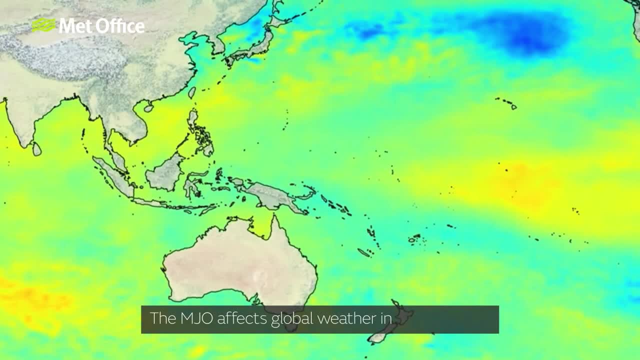 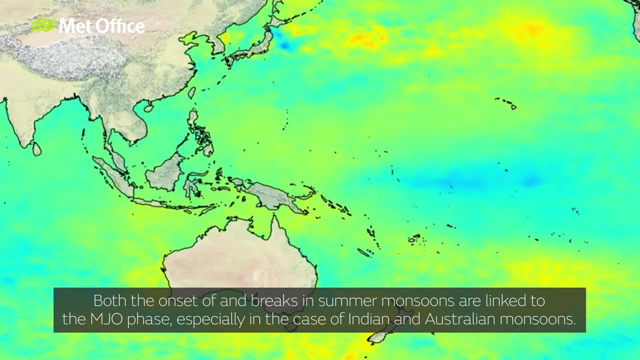 eventually dying out in the Central Pacific. The MJO affects global weather in several ways. Both the onset of and breaks in summer monsoons are linked to the MJO phase, especially in the case of the Indian and Australian monsoons. There is also a strong link between the MJO phase and tropical cyclones. 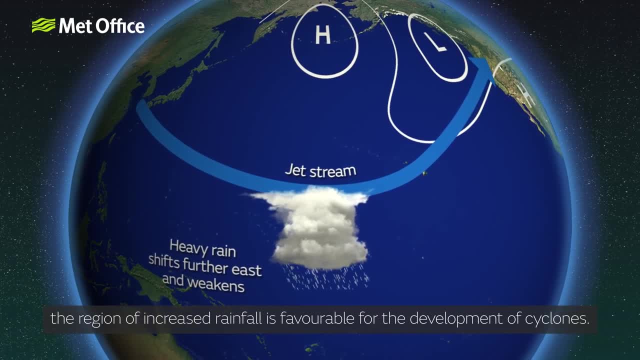 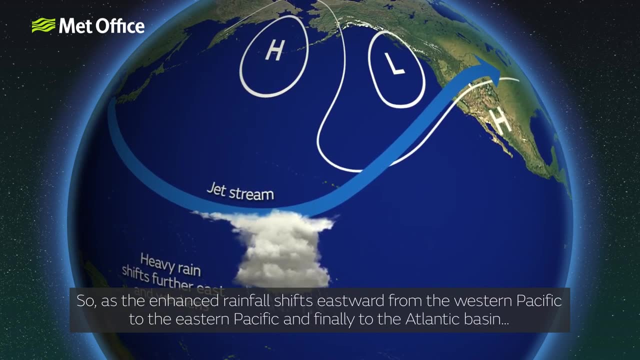 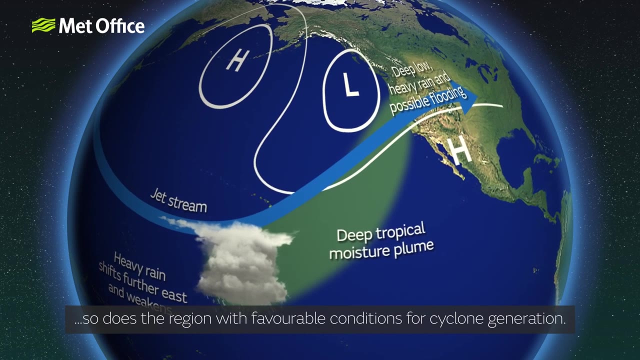 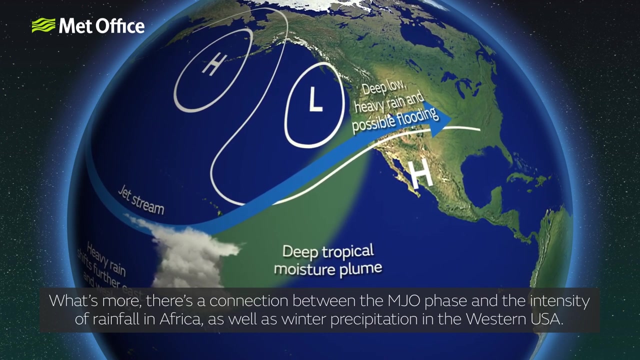 The region of increased rainfall is favourable for the development of cyclones, so as the enhanced rainfall shifts eastward, from the Western Pacific to the Eastern Pacific and finally to the Atlantic, So does the region with favourable conditions for cyclone generation. What's more, there is a connection between the MJO phase and the intensity of rainfall. 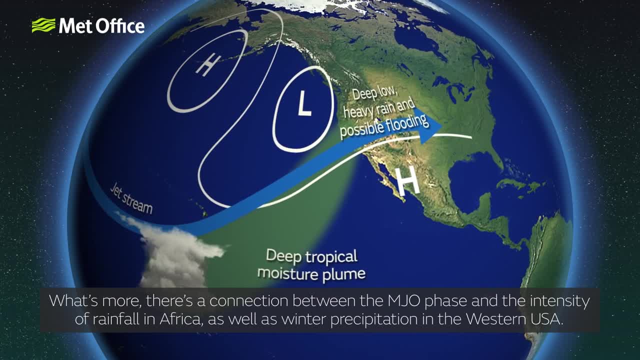 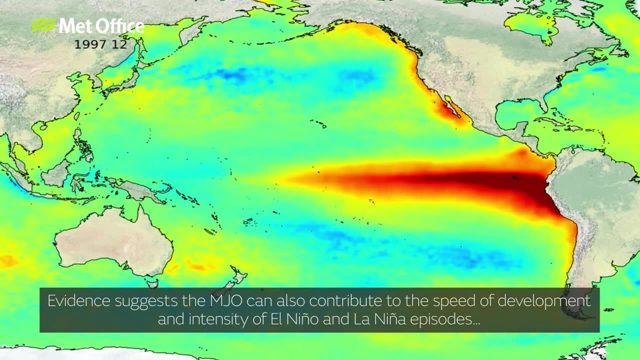 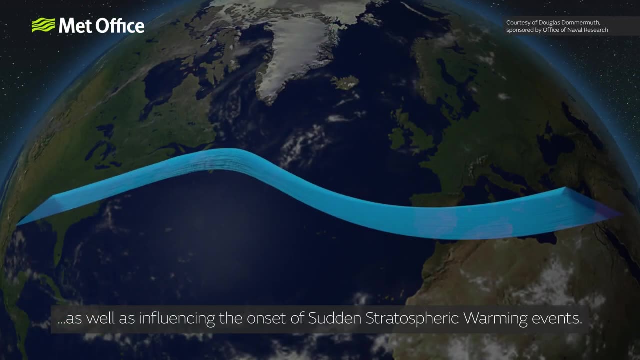 in Africa, as well as winter precipitation in the Western USA. Evidence suggests the MJO can also contribute to the speed of development and intensity of El Niño and La Niña episodes, as well as influencing the onset of sudden stratospheric warming events.